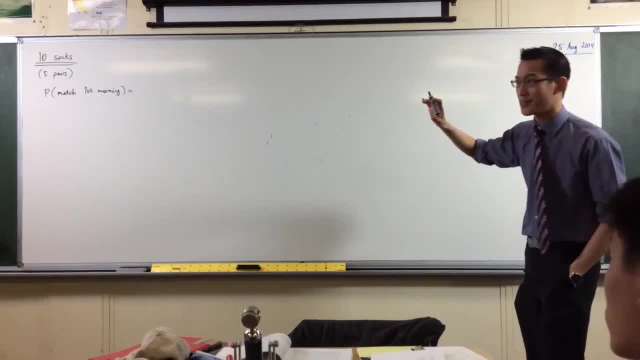 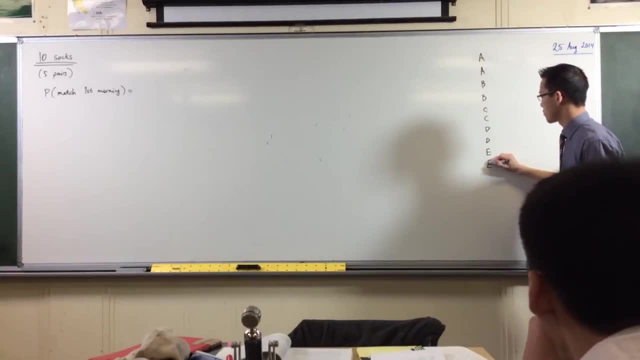 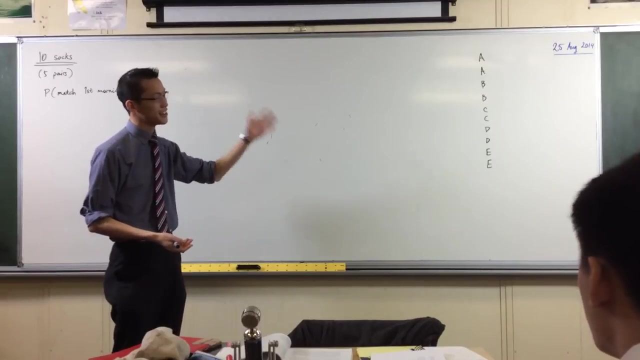 And I'm just going to write out over here. I don't have five colours, so I'm going to write them just as of different letters. Okay, So here are my ten socks: five pairs, right, Five different colours letters. you get the idea. 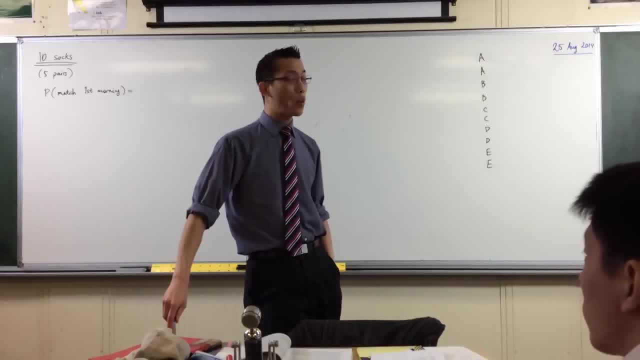 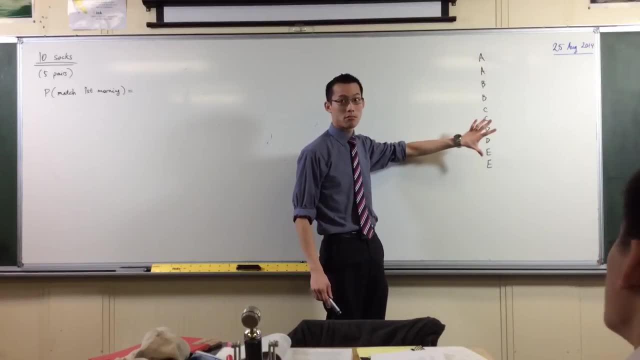 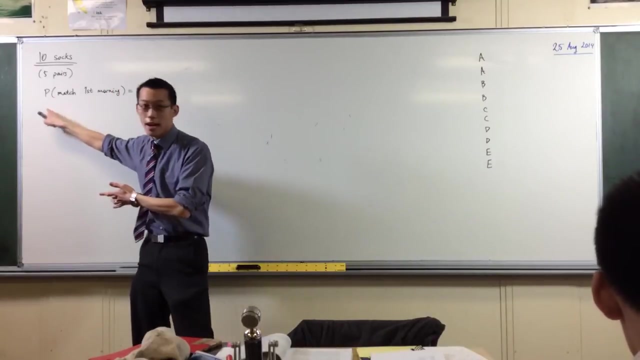 Now think about that first sock. Does it matter which sock I pick, Like, do I want a particular sock over any other one? No, it doesn't matter, right? So the way I can think about this is being that this is all about probability, right? Probability. 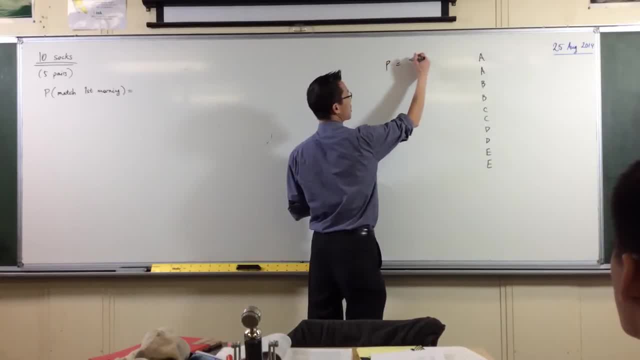 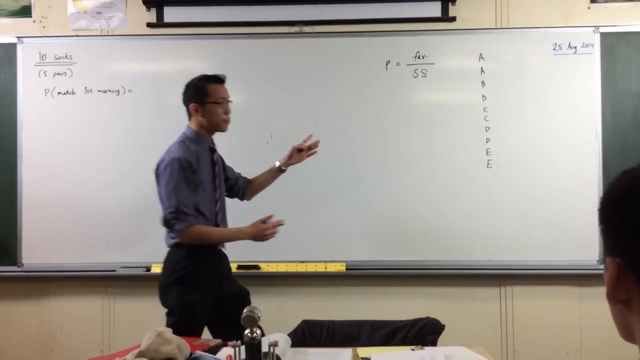 And probability is a fraction. Probability is always a fraction of something over something. What are the two things? It's favourable outcomes, right. Favourable outcomes, the ones that you want over sample space, right? Okay. So being that my sample space, clearly that's ten, right. 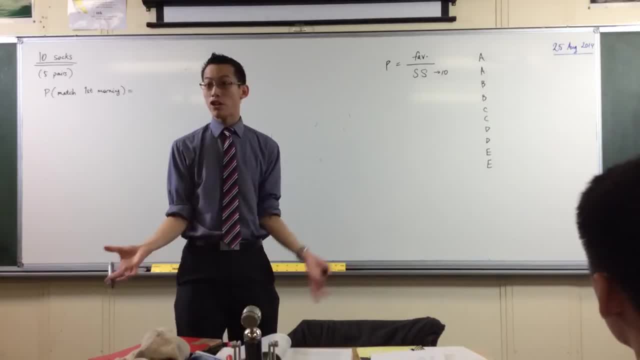 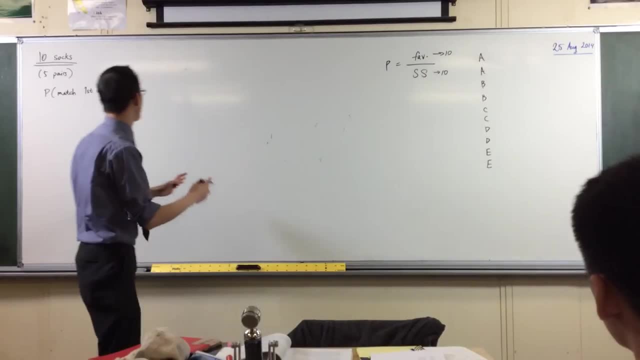 But when I ask you, like: which sock do I want? Well, we don't care which one, They're all good at this point in time, right? So the favourable outcomes is ten, right? So the first thing I'm going to write is one. 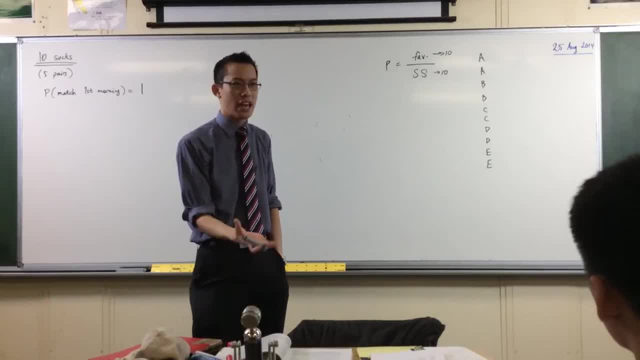 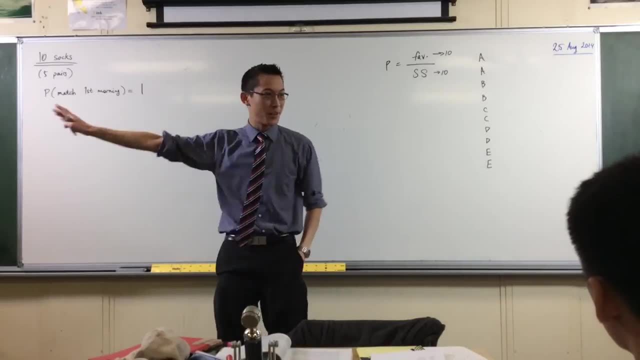 Now you might think: well, why are you writing that? That's not going to change the answer? No, it's not, but it's meaningful. right, As you will see, capturing all our meaning in the working out that we do is critical. 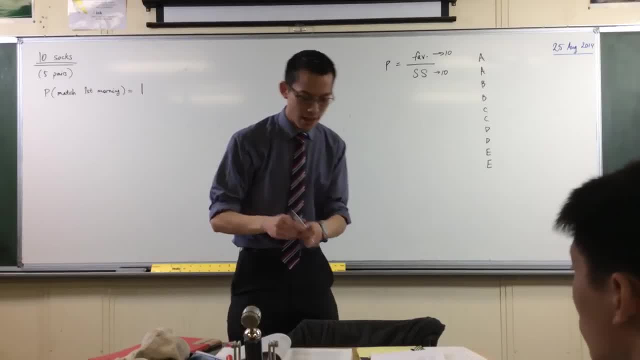 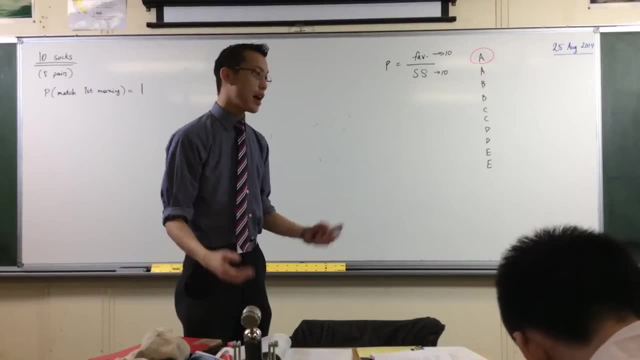 It starts off easy, but it gets trickier later on. So I pick a sock. okay, Let's suppose it's this one, right? First sock down, And then I have to pick another one, and I want a match. 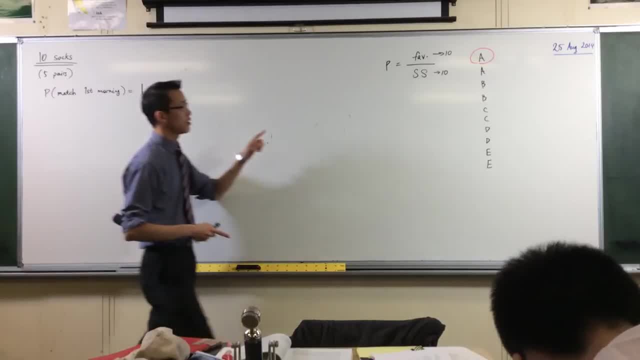 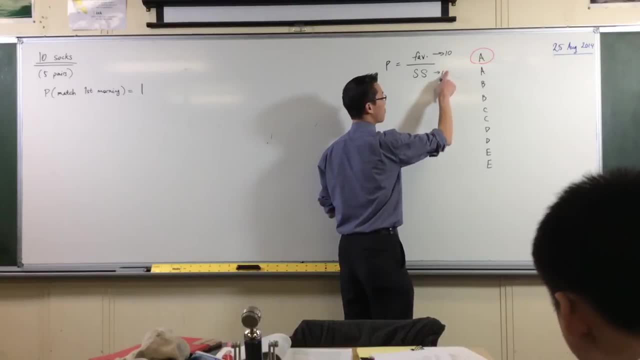 That's what I'm after, okay. So two things have changed. Firstly, the sample space has changed. right, I don't have ten socks anymore, I have nine, Right, So that's reduced, okay. But also now that I have one of the socks in particular, 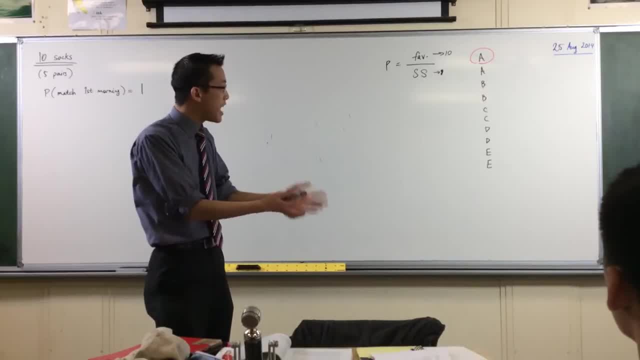 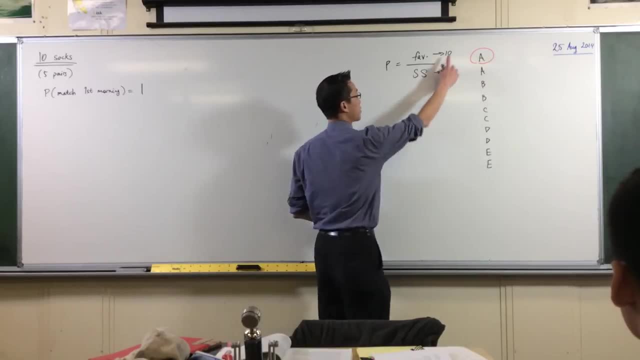 the favourable outcomes has also changed. right Now that I've picked one, the second one, I only want this one. This is the only one I'm interested in. Yes, Okay, So far, so good. So the probability of getting a match after that second sock will be: 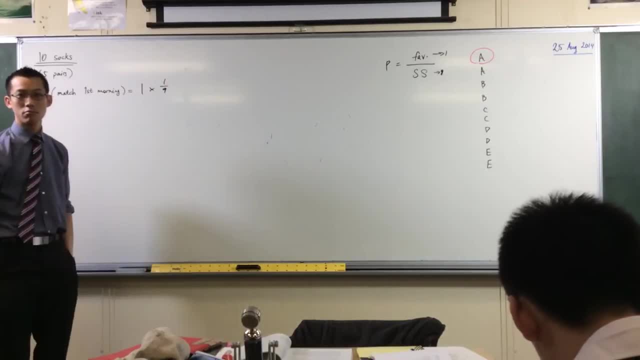 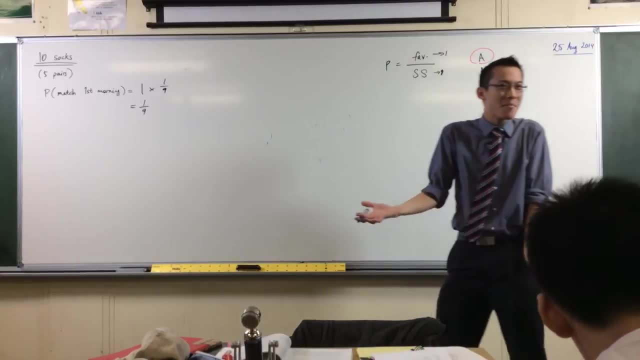 One times one over nine. There you go. okay, That's one over nine. There's the probability. Not so bad, right? What's so hard about this question? Well, let's progress Now. they give you a whole variety of different mornings. 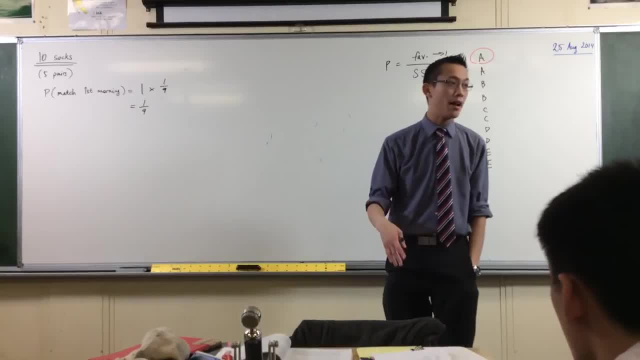 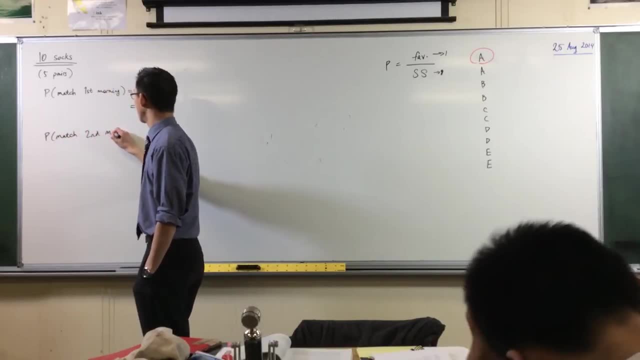 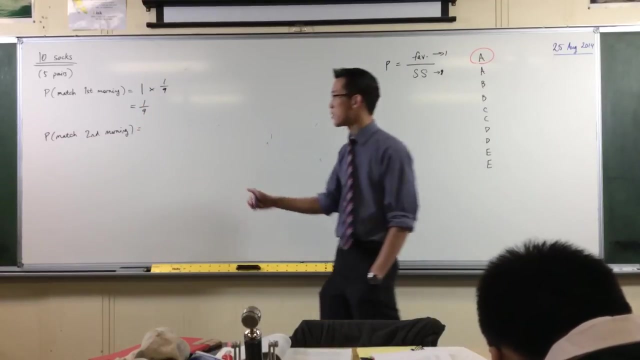 To make it easier to illustrate, I'm just going to think about the next day. Twenty-four hours passed and now I'm thinking about getting a match the next day. Okay Now, keep in mind this is quite separate to what happened before. 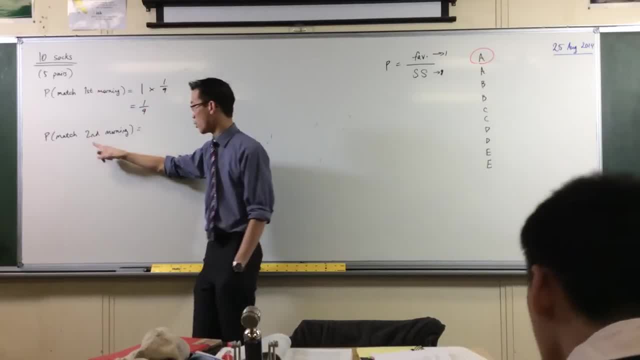 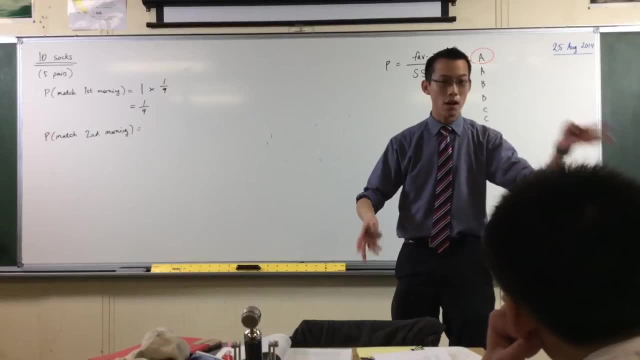 I'm not thinking about a match the first and second morning. I would have written first and second morning here, not two matches in a row. Just forget about what happened the previous day. I might have got a match, I might not have. 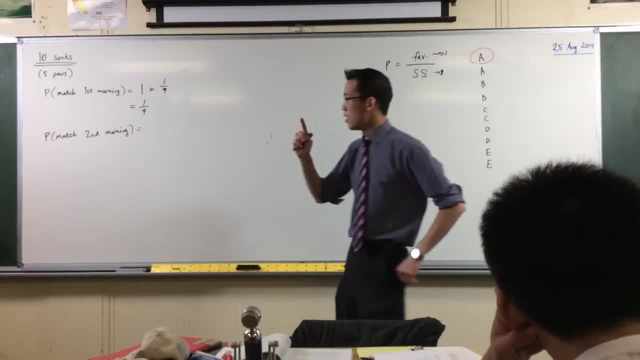 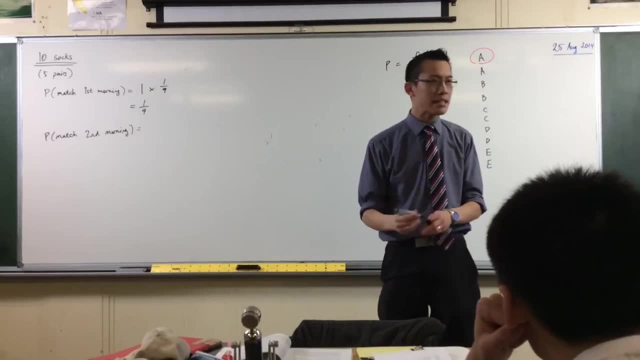 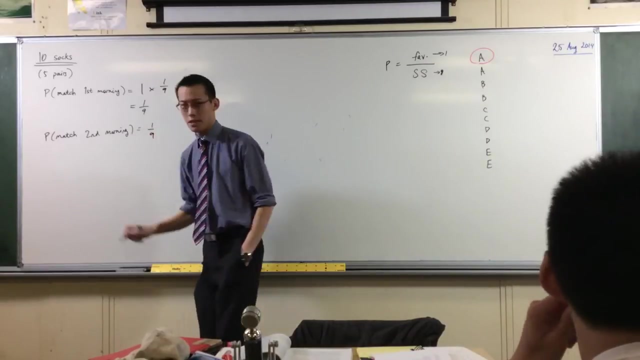 I'm just interested in Tuesday: Okay, What's the probability of getting a match now? Okay, Now, who has an answer that jumps out at them? Any thoughts? One over nine? One over nine? Okay, One over nine Now, how many people agree with that? 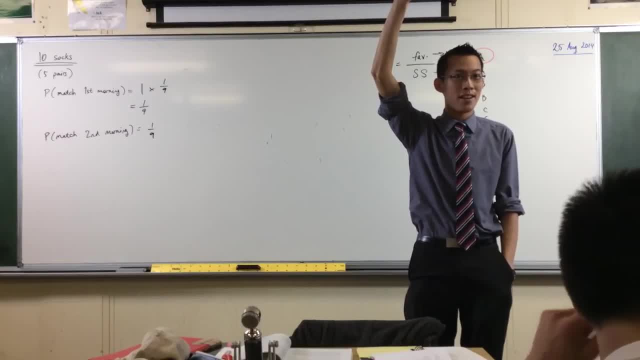 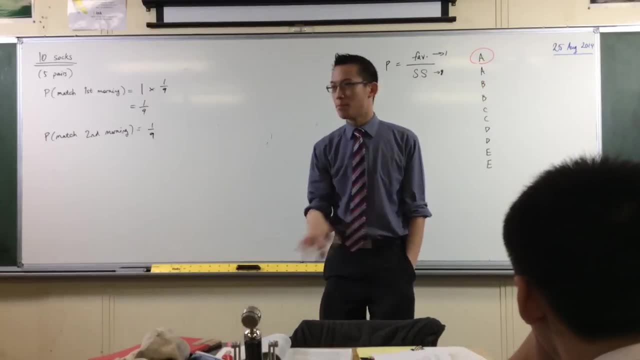 You don't have to provide an explanation. I'm just interested in who thinks that's a plausible answer. Hands up straight. I actually want to see: Okay, All right. All right, Put your hands down. Everyone who didn't put their hands up just now. I want you to raise your hand for a second. 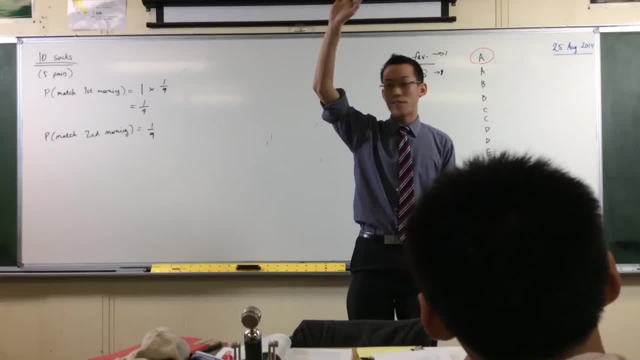 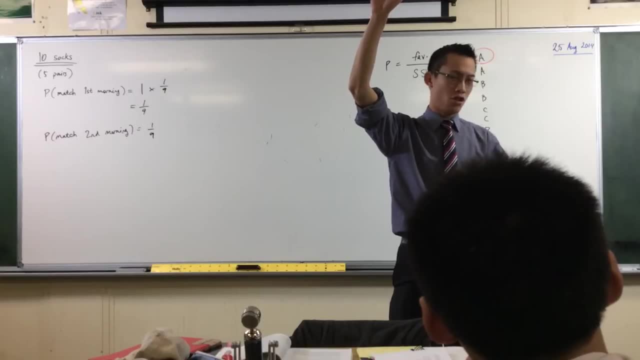 Okay, Now I want you to keep your hand up if the reason you don't think it's one over nine is because you think it's something else. Do you think it's something else, Or do you think it's something else? Put your hand down if you're just not sure. 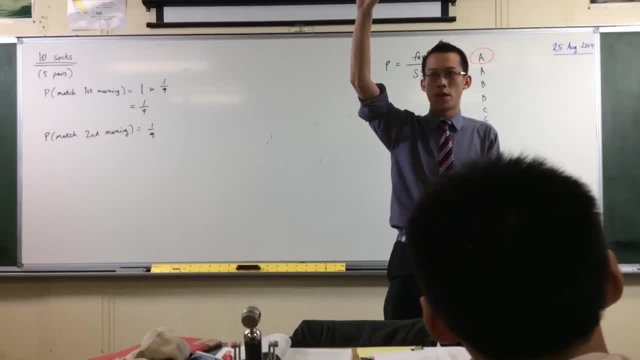 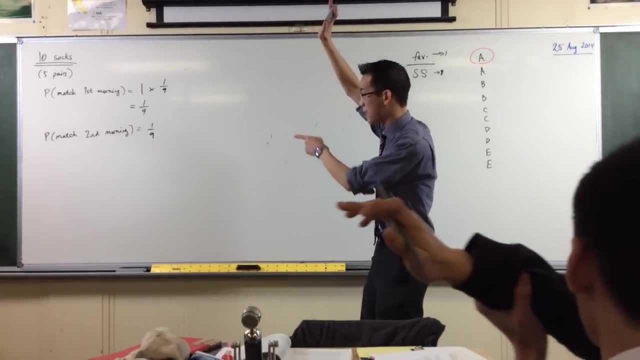 But keep your hand up if you think it's something else. It can't be one over nine Hands up. Okay, Now anyone who's still got their hands up, because, by the way, I have my hand up. I think this is weird. 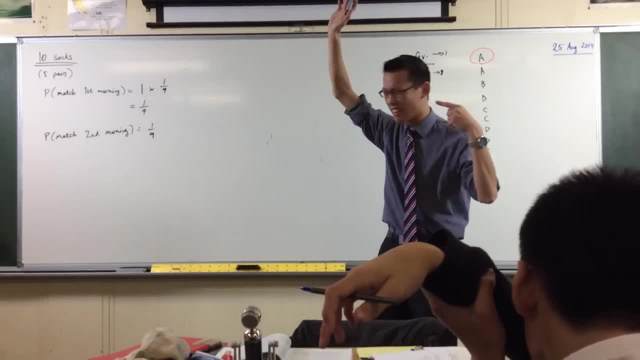 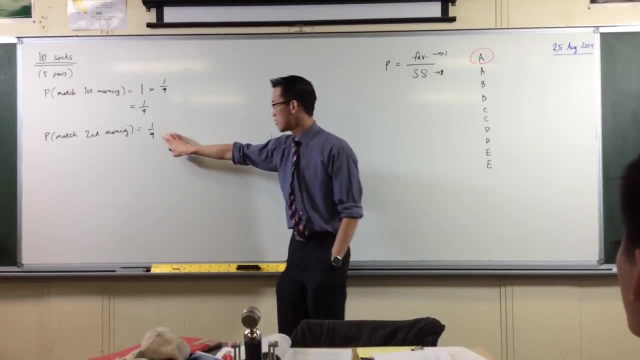 I think this is very strange. My intuition is kicking in and saying: really, Anyone who's got their hand up why You can put your hands down now, But why you guys who did have your hands up? why do you think this seems strange? 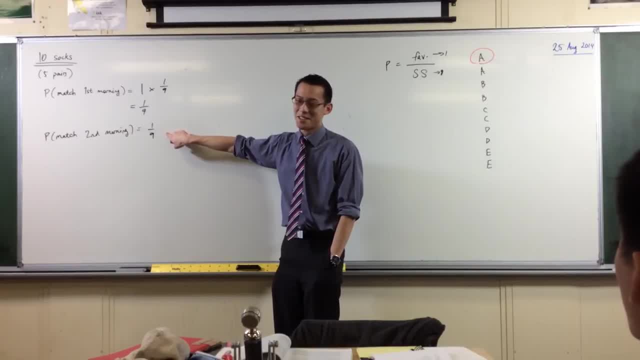 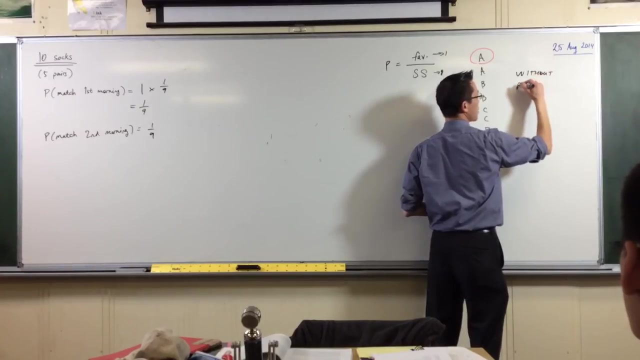 Why do you disagree? He has to wash his socks. He has to wash his socks, Okay. So what difference would that make? Okay, All right. So you're saying this whole scenario, this scenario is without replacement. Now hold on a second. 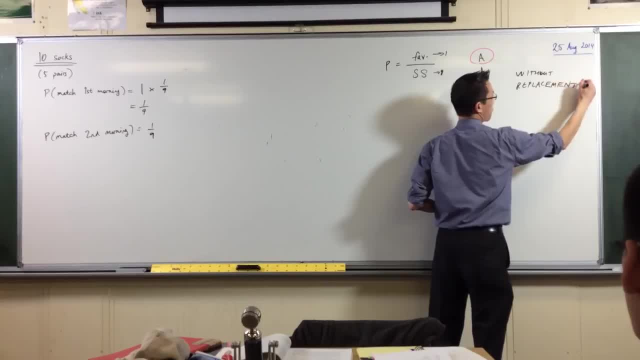 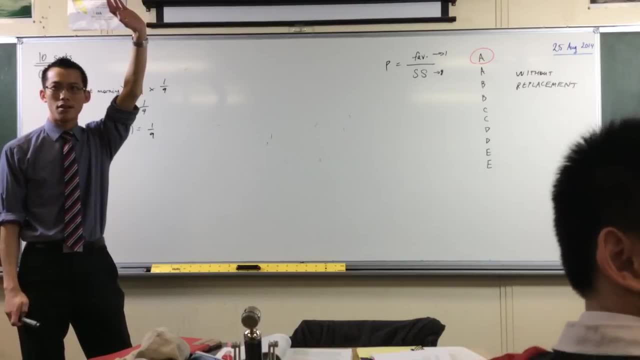 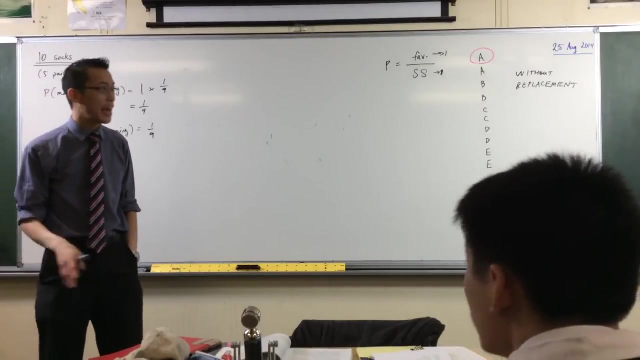 Before we leave off this: who thinks Elion is right? Who agrees this situation is without replacement- Okay, Hands down. Who thinks it is with replacement- Okay, Hands down. I know a few of you don't know, That's okay. 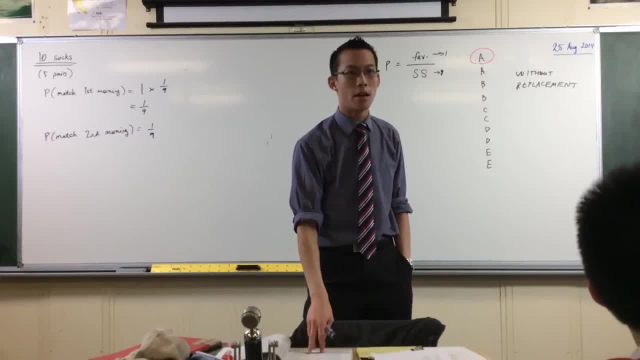 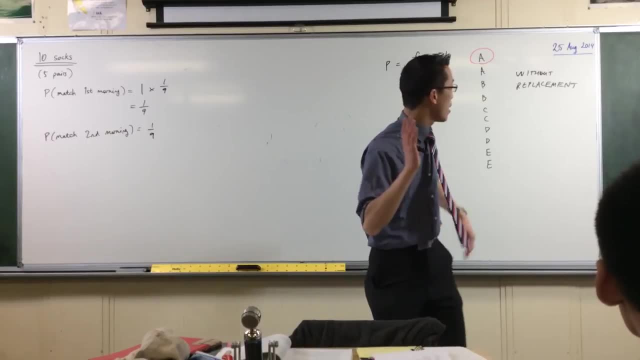 Look at the question again. Look at it carefully. Read it with me. It's all in the language. Is there anything in the question that suggests to you it's going to be with replacement or without? I think Elion's right, I think it's without replacement. 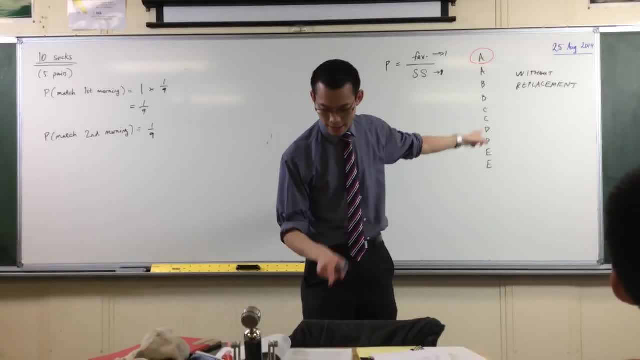 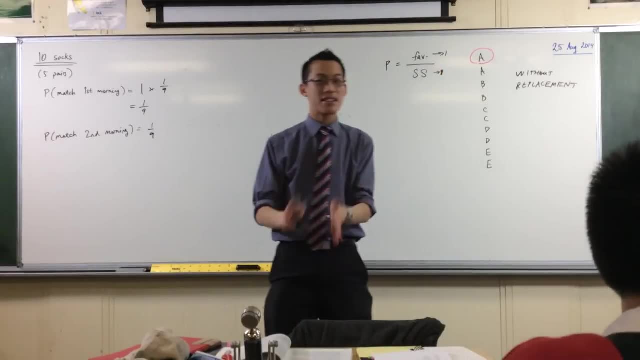 And I think the key word is he has five different pairs of socks to last the week, which kind of implies by the time he gets to Friday he's pulling the last two socks out of the drawer Without replacement. I think is correct Okay. 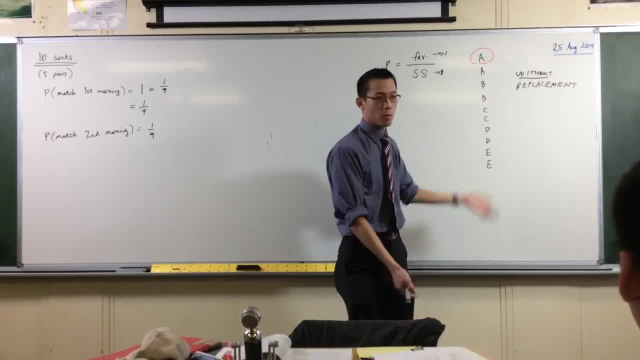 Now hold on. Let's keep pushing on that. If it's without replacement, why is that a problem? Why does without replacement suggest to you that this answer has a four in it? Because you would think by the next morning, just like you know, when we looked at the 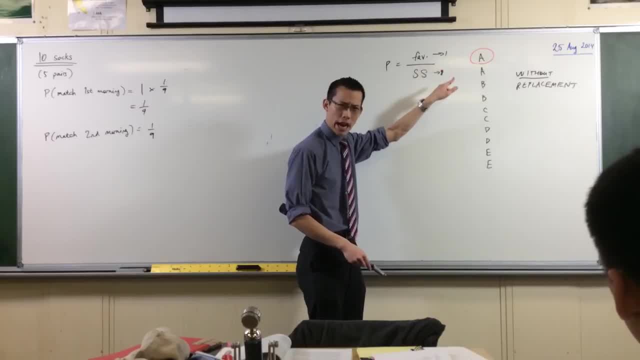 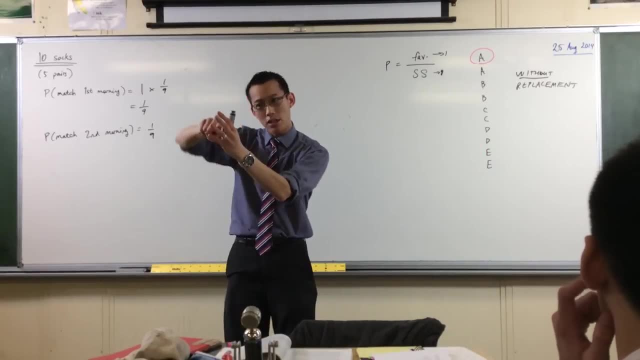 first sock and then the second sock, the sample space would change, right. And we looked at this yesterday. We looked at the idea of dynamic probability, where when one thing is correct, the other thing depends on the previous thing. then the probability changes every time. You would. 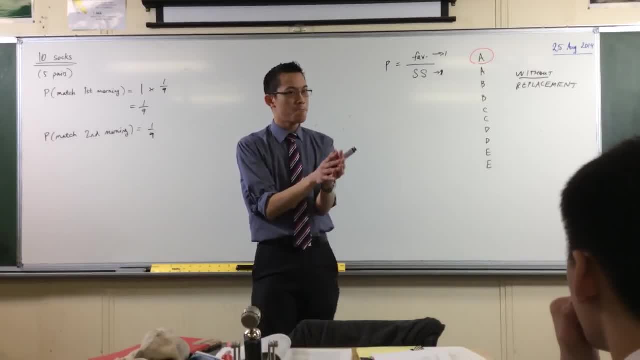 think the second morning and the third morning and every subsequent time, probabilities change, right. So I agree, I agree that something seems suspicious with this. Now the question gives you a clue Right at the beginning. I didn't read this. It says this question: 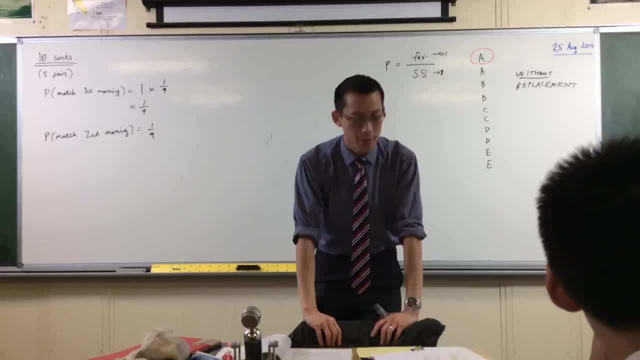 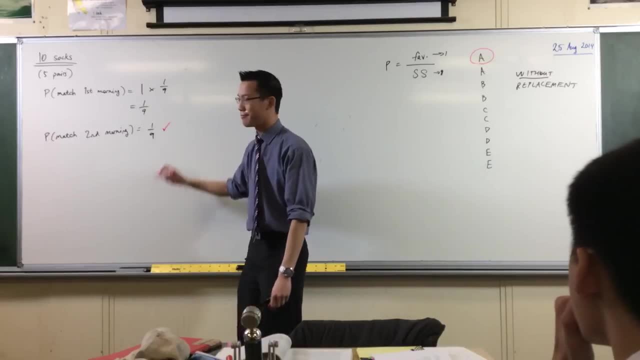 and the next are best done by retelling the story of the experiment. Now what happens is you go to the answers, okay, And you look for this and you find, sure enough, a 9 actually is correct, And then they give a bit of an explanation. Now their explanation goes like: 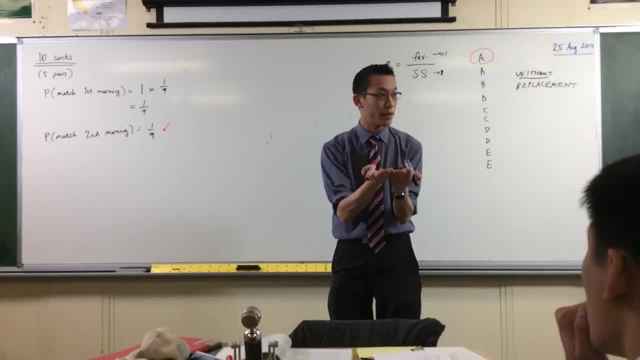 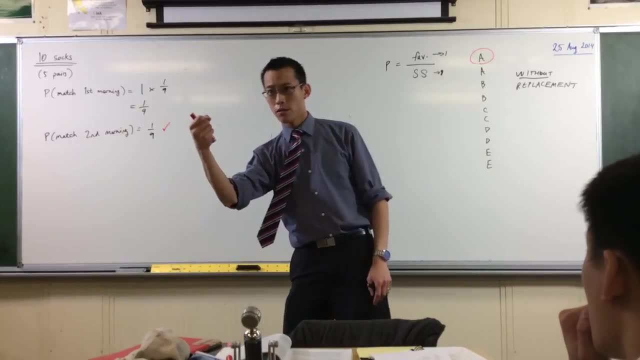 this. They say they follow the advice. They say: retell the story. okay. So what they imagine is: well, you know how I walked through this. I said: okay, the first morning I pick out this one, and then I pick out this one, right, Well, let's retell it, Let's retell. 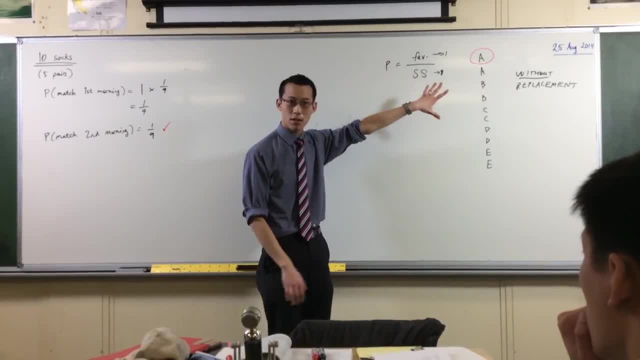 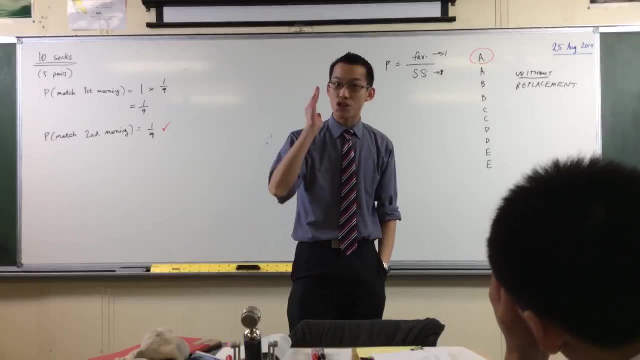 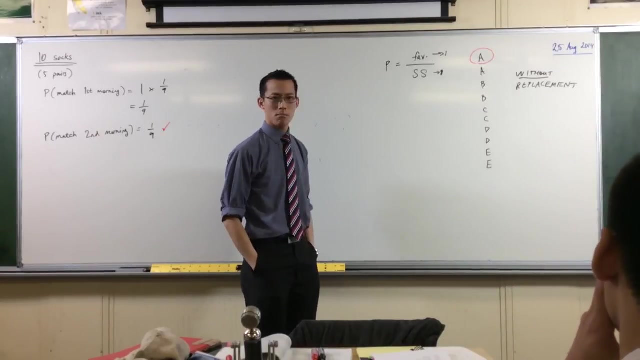 it like this: okay, It's Monday morning, I have 10 socks in the drawer. Okay, But instead of getting out Monday's socks on Monday morning, I get out Tuesday's socks on Monday morning. Now, what has changed? And the answer is: nothing has changed. I'm